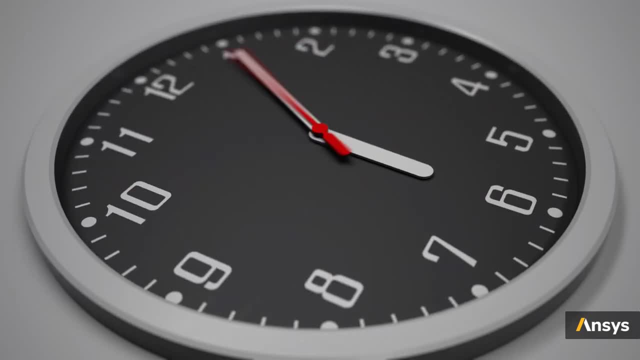 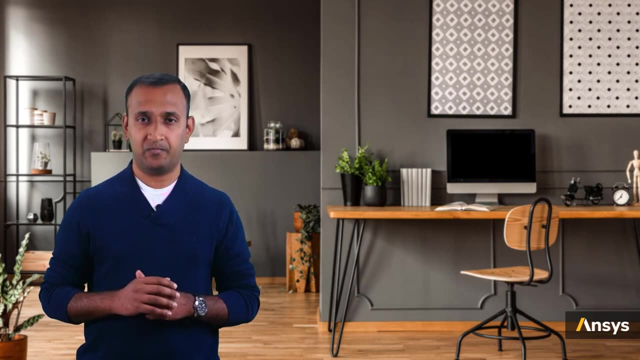 nothing but a time domain analysis or a transient analysis. But it's not always necessary that we study a system's behavior over a time. So how do we decide a need for a time domain analysis and how do we assess the time range over which we need to analyze a system's behavior? 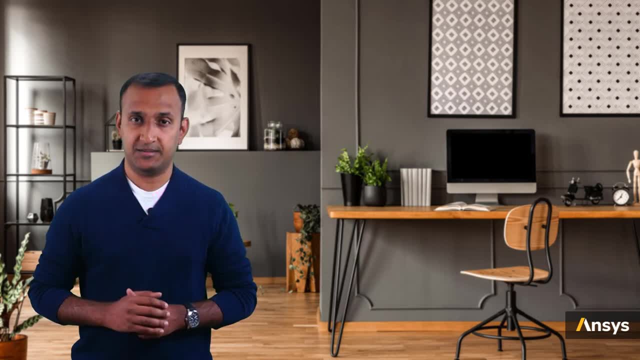 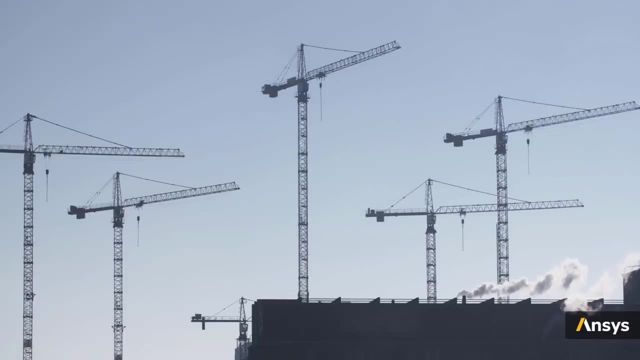 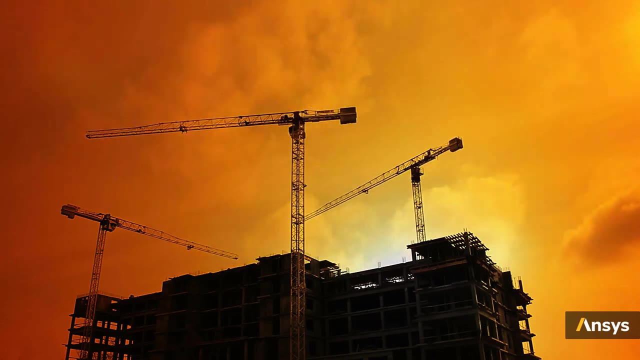 This boils down to the physics that's related to the set changes. From an engineering standpoint, sometimes we are only interested in the system's behavior after it achieved a state of equilibrium, and sometimes we are interested to know what happens to it while it is achieving this state. 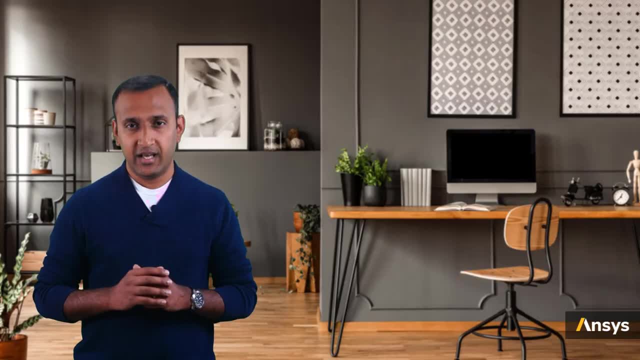 of equilibrium. Either way, it's important for a good engineer to identify the physical phenomena that are changing a system's behavior and then study them for an appropriate amount of time. In this section, we'll discuss the primary reasons that bring about a time-dependent behavior in mechanical systems that an engineer 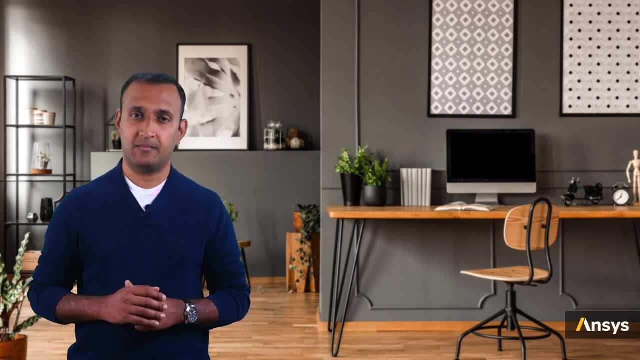 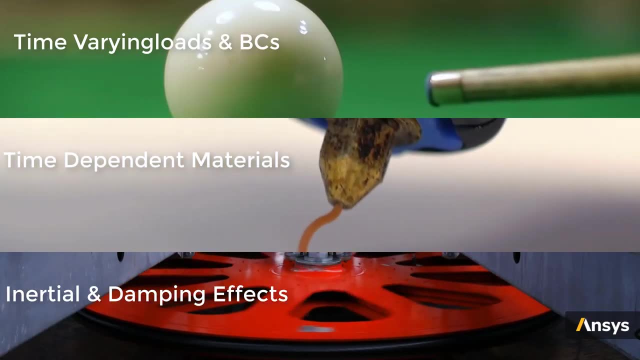 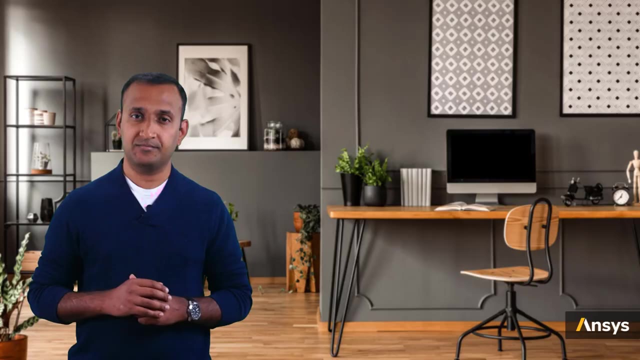 must consider in their design process. We'll focus on three aspects, namely time-varying loads and boundary conditions, time-dependent material behavior and inertial and damping effects. Let's look at a few examples of each of these types to better understand the 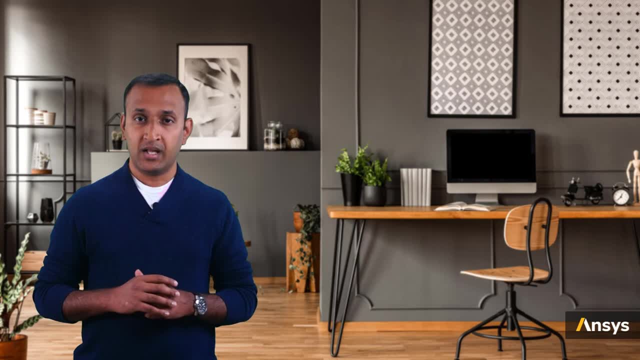 how they make mechanical systems time-dependent and how a time domain analysis can help us analyze them. We'll start with a very common occurrence, which is time-varying loads and boundary conditions. We see this everywhere and every day. For instance, if we place our smartphone on the 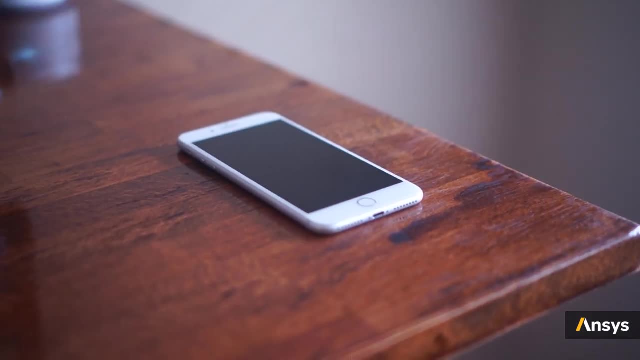 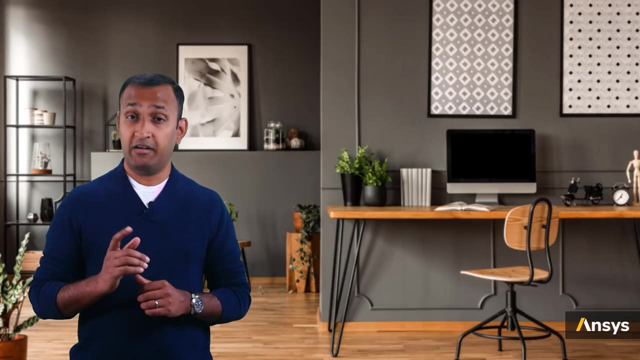 ground, then the weight of the phone is the only load that is acting on it and it is acting gently. If we drop the same phone from a certain height upon its impact with the ground, its weight is still the only load that is acting on it, but it acts rather abruptly or over. 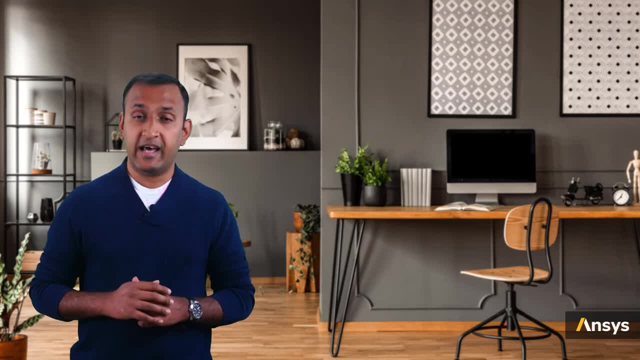